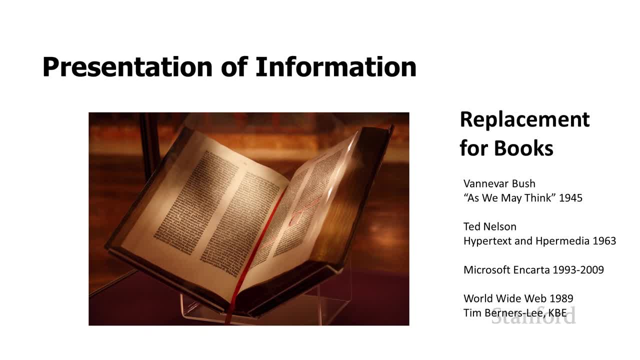 found on CD-ROMs. Microsoft and Carta, starting in 1993, provides a really good example of this use of technology, And the World Wide Web first came out in 1989, which, you'll note, actually precedes Microsoft and Carta. 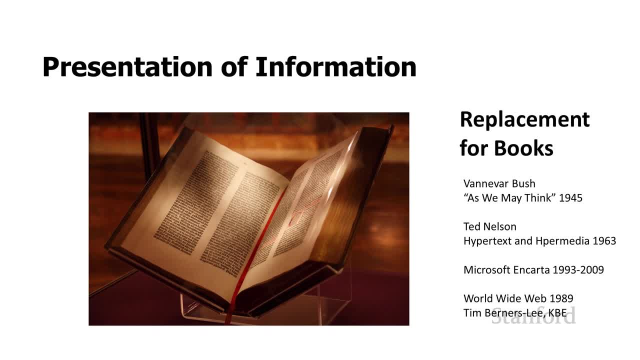 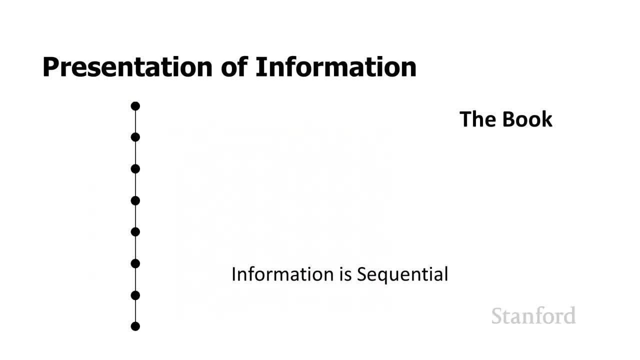 But it was only in use by a very limited number of people, And we'll be taking a look at that in a couple of minutes. All right, so what's wrong with the book? Why would we want to replace it? Well, one thing about a book is it's a book. 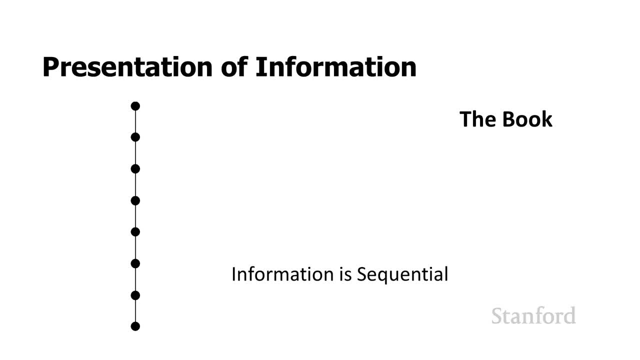 A book consists of pages and each of the pages follows a preceding page sequentially. I mean that's fairly obvious, but it turns out this can be a pretty big limitation. It really depends on what sort of book we're looking at. So we have page one followed by page two. 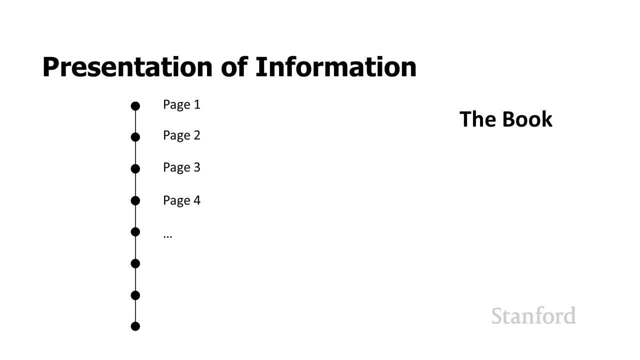 followed by page three and so on, And we're reading fiction. This is probably a good choice, unless, let's say, it's a mystery novel and you just can't handle waiting until the end, and so you flip to the end to see what's going on, or possibly. 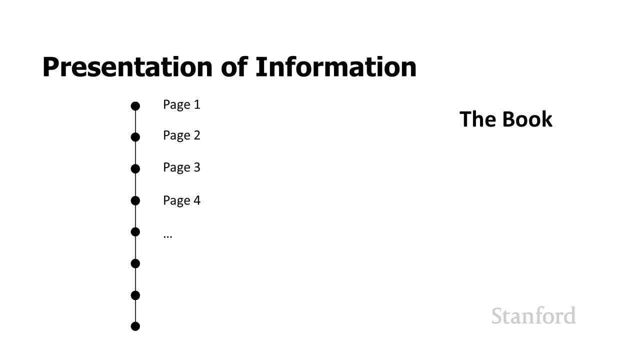 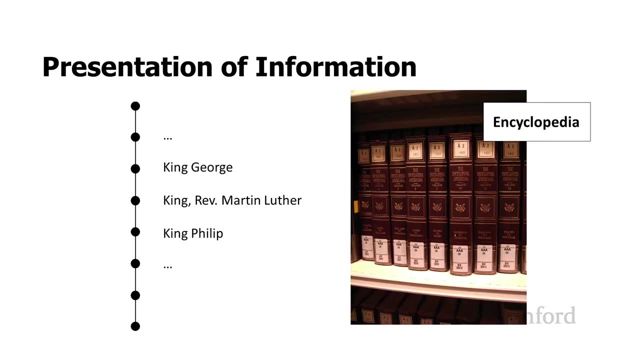 you're a literary criticism major and you want to jump around the book, But most of us are perfectly happy with the linear nature of fiction novels. In contrast, think about something like an encyclopedia, Because an encyclopedia is printed, it's got that single sequential information flow. 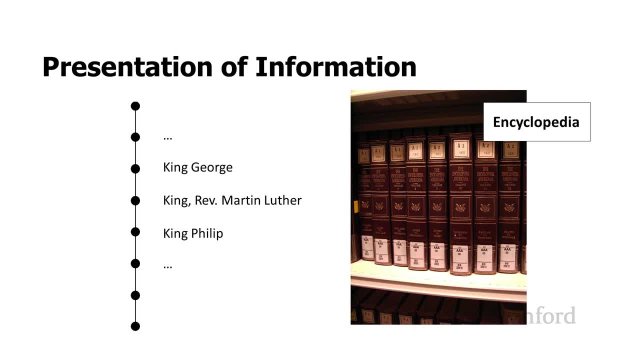 So if we're looking for an article on the Reverend Martin Luther King, we're likely to find him sandwiched between King George of England and King Philip of Spain. What does he have to do with those two? Well, the encyclopedia only has one ordering of information. 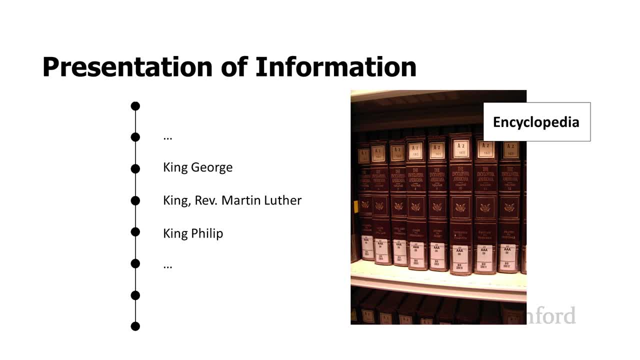 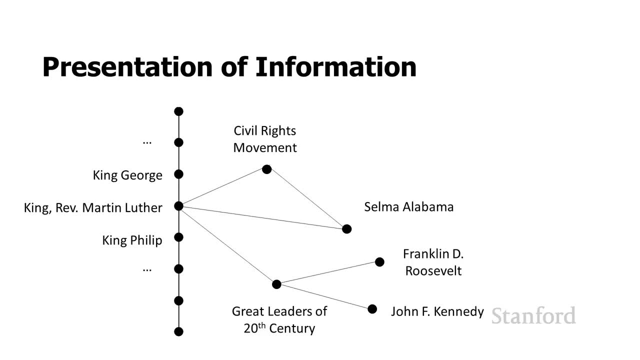 and it uses that linear ordering of information to make it easy to look up articles, not to find links between different articles. And so when we move to computers, we're no longer limited to that single ordering of information. We can create different nodes of information. 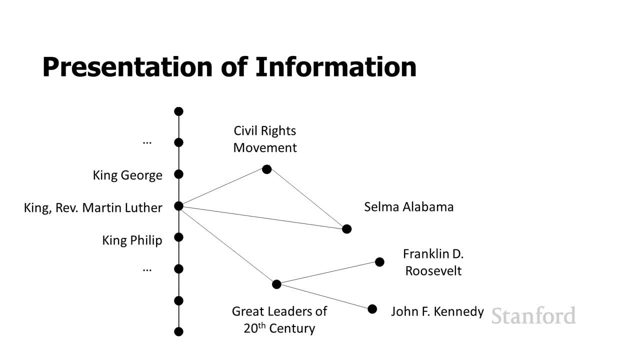 and link any node to any other node. So we can still maintain our sequence of information for lookup if we wanted to. but we could also link the Reverend Martin Luther King to articles on the Civil Rights Movement, to Selma, Alabama, to the great leaders of the 20th century and so on. 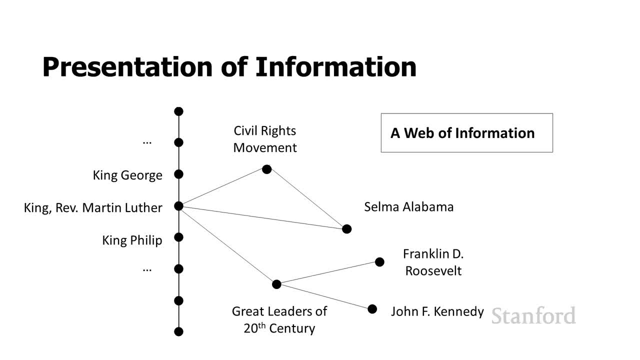 We now have a web of information, which is where the term World Wide Web comes from, of course, And this concept of hypertext basically said that we have these different text nodes and that we're going to link the text nodes And, of course, this is exactly how the World Wide Web works. 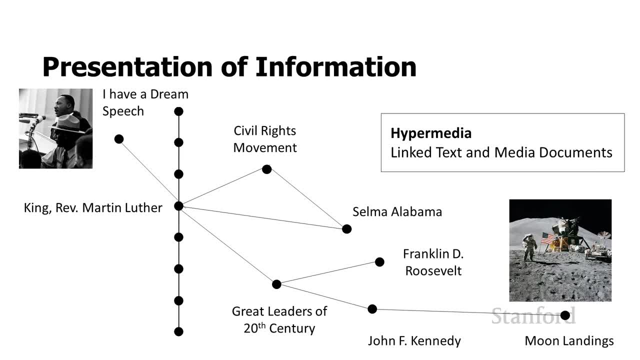 We can take things a step further on the computer, because we're no longer limited to just text. We can have Speeches, we can have audio, so we can have the Reverend Martin Luther King's- I Have a Dream speech. We can have photographs. 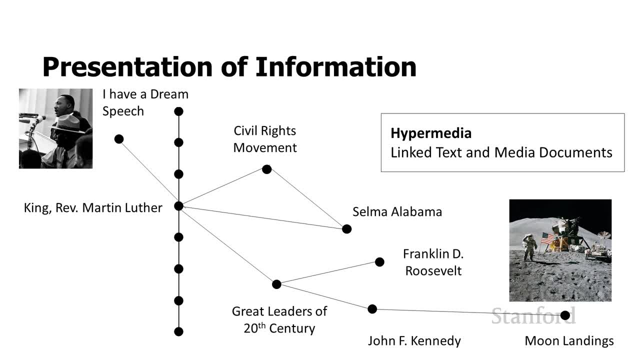 We can have movies, And so this is called hypermedia. OK, so that's the basic idea behind hypertext and hypermedia, But that still doesn't get us to the World Wide Web yet. That's only half the equation. We've seen that the other half of the equation is the internet. 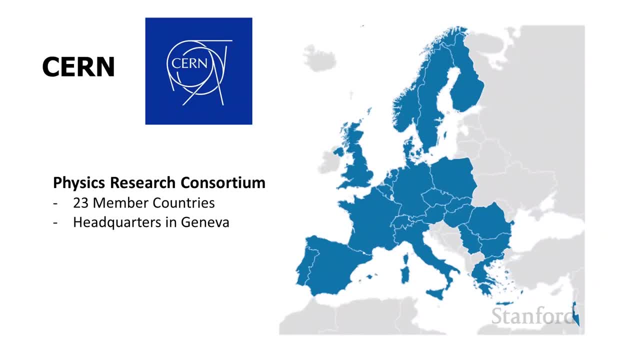 but how did the two end up together? Well, we need to move to Europe, and in Europe there's a physics consortium called CERN. It has 23 member countries and its main headquarters in Geneva. It's most famous for a large collider, which. 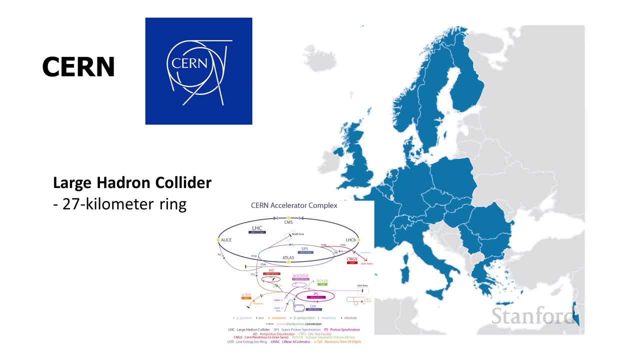 is used for high energy physics, Not that different from our very own Stanford Slack, And in this case they have a 27 kilometer ring which is used for high energy physics and smashing particles into each other. Now, in the late 80s, one of the computer scientists 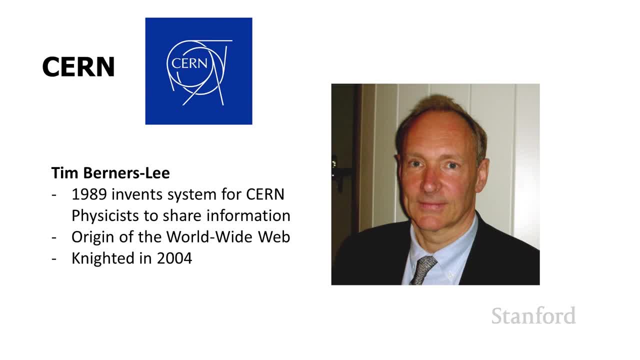 working for CERN was interested in coming up with a way for the physicists at CERN to share research papers. One of the things that happens at CERN is the member countries send their physicists to CERN and then sometimes they return to their own institutions. 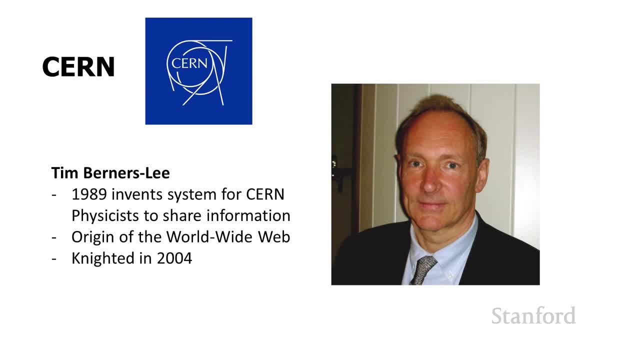 in their various countries, And so he was looking for a way to share papers between all the physicists, And naturally he thought we should use the internet, But, in addition, he thought we should use that hypertext technology that people have been talking about. 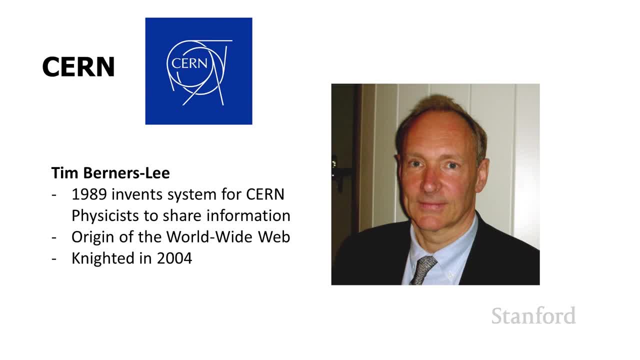 and it's been sitting in the research lab for quite some time And nobody's actually Using. If you hear some tinkling in the background, that is actually Maddie drinking from her dog bowl and her dog tags hitting the dog bowl. Anyway, so Tim Berners-Lee in 1989.